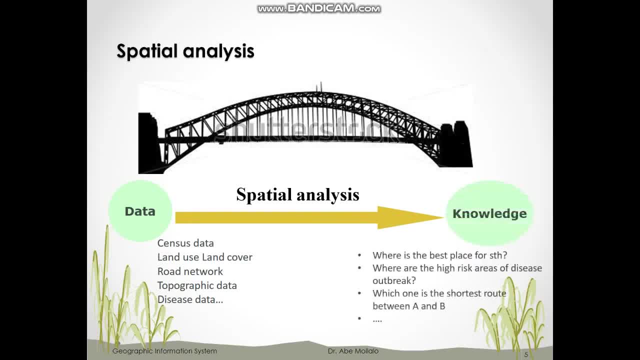 we saw the robot application, the, desseing the data to make the data available to the individual. but not just the model model, but also uh systems. The next step is to combine this data and turn the data into knowledge to solve real words problem. 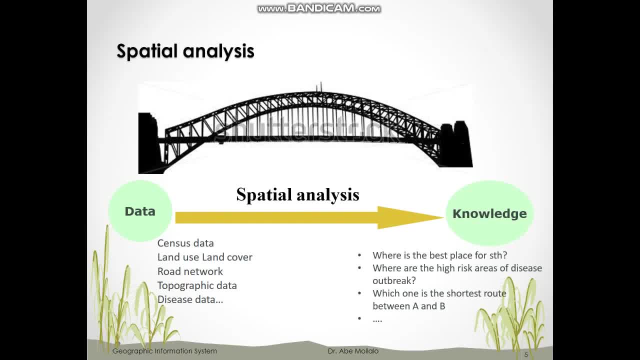 For example, where is the best place to build the new hospital based on several criteria- Uh factors like slow, proximity to high population, proximity to road should be combined- or Where are the high risk innovative data available with a FTO model 7? Jeff, your bar is over there. Les and James can answer your questions in six minutes. 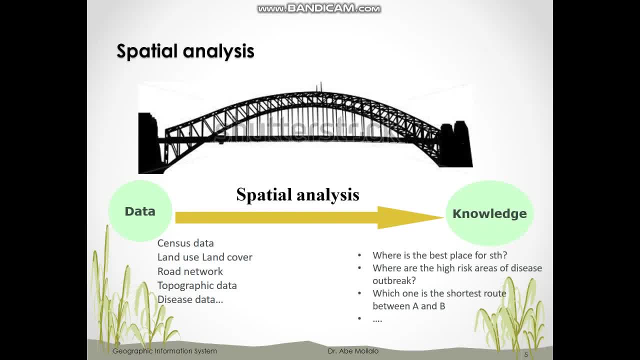 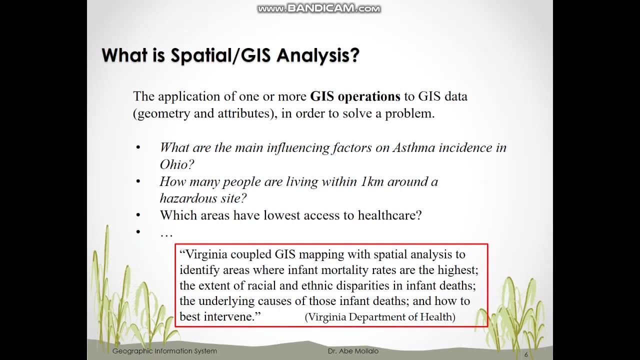 areas for disease outbreak. we can allocate resources, budget, to these areas to control the outbreak. which route is the shortest route between your house to the university? so these are knowledge that we can extract from the data. so what is the spatial analysis? technically, spatial analysis is the application of one or more gis operation in order to solve real world problem, such as what? 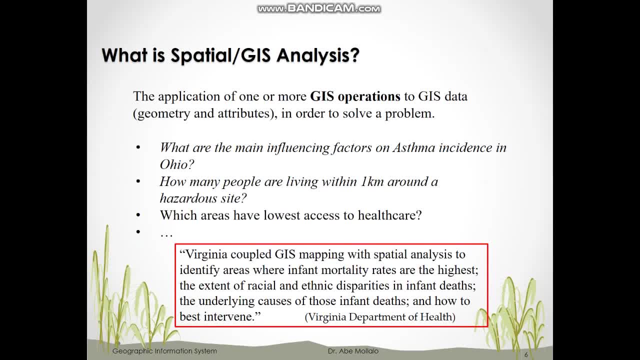 is the shortest path between your house and department by car? how many people are living within one kilometer around the hazardous site to risk assessment or? or health disparity: which areas have lowest access to health care or another real world application in public health? according to virginia department of health, is virginia coupled gis mapping with spatial analysis? 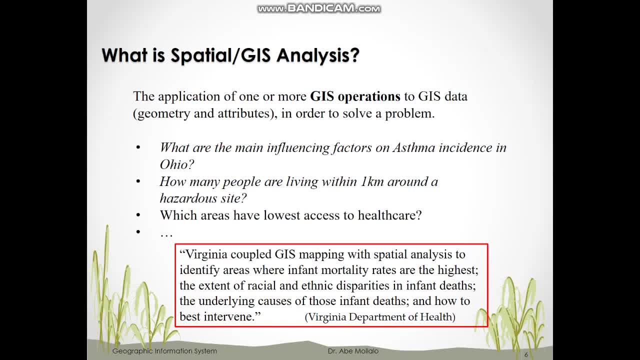 to identify areas where infant mortality rates are the highest, the extent of racial and ethnic disparities in infant deaths, the underlying causes of those infants and how to best intervene. so these are knowledge you can extract from the prepared data to support your decision making, to make decision based on the fact. 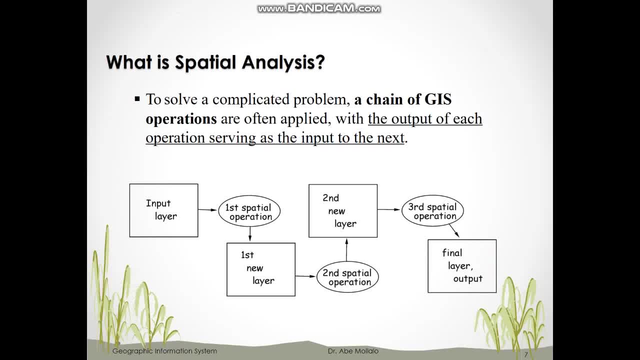 technically, a spatial analysis is a chain of gis operations. a chain basically means the output from one gis operation is served as the input of the second gis operation, and so on. so operations are linked together to solve the real world problem. so here, for example, the input layer, we have a input layer. a spatial analysis is done on the input layer. so 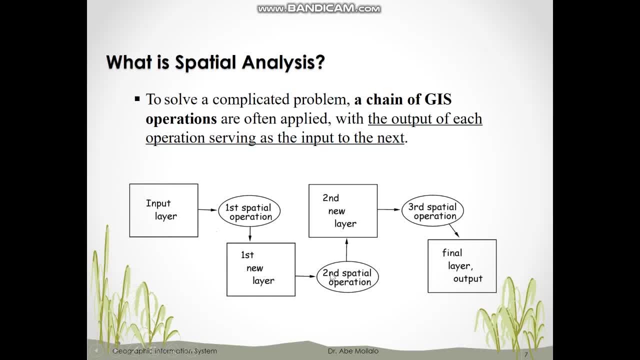 we will have an output layer. the output layer will be the input for the second spatial operation and gives us the output layer, and this output layer serves as input for the spatial operation and gives us a final output layer. so you can see, in the the operations are linked together to solve the real-world problem and by 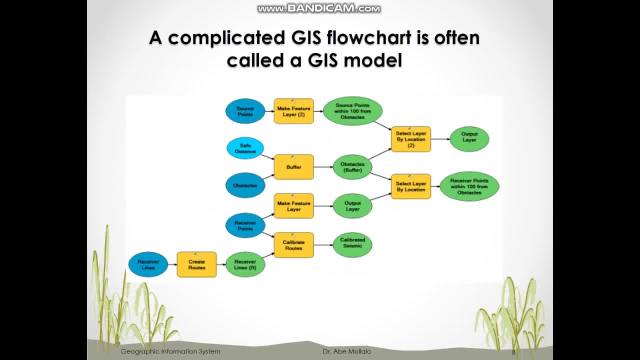 chaining GIS operation. you will have a complicated GIS flowchart like this and a couple of input layers with many GIS operations linked together. it is called a GIS model. in the future lecture you will build sophisticated GIS model in ArcGIS and solve complicated real-world problems that are not easy to solve. 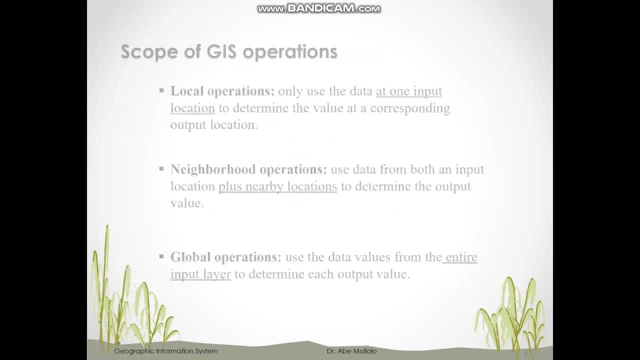 without GIS. so basically there are three categories of GIS operation which we will talk about a little today. we just scratched the surface and with more details in the future lectures. so GIS operations can be divided into three categories: local operations, neighborhood operations and global operations. local operations basically mean the output is determined based on the input in 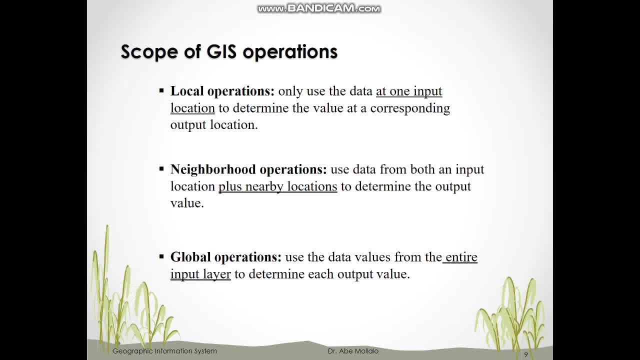 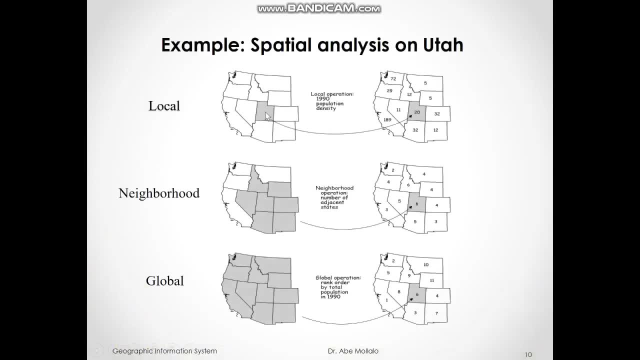 the same location. so or input and output are for one location. for instance, this gray polygon is the state of Utah. we want to calculate population density of this state and the output here only depends on the population size and also the area of the state. so we only need information about Utah State to calculate. 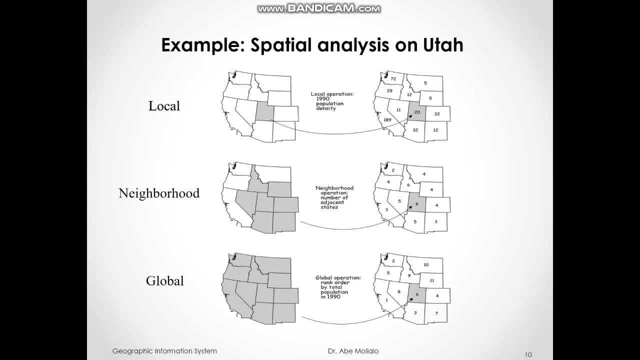 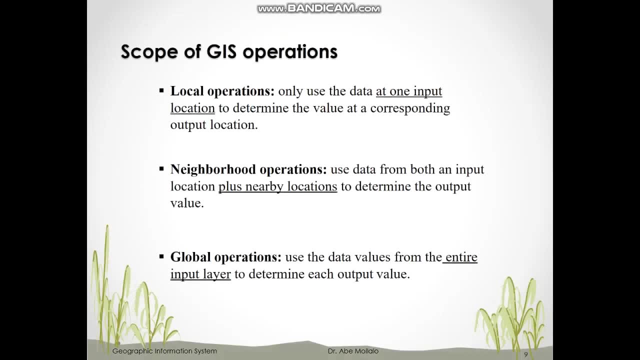 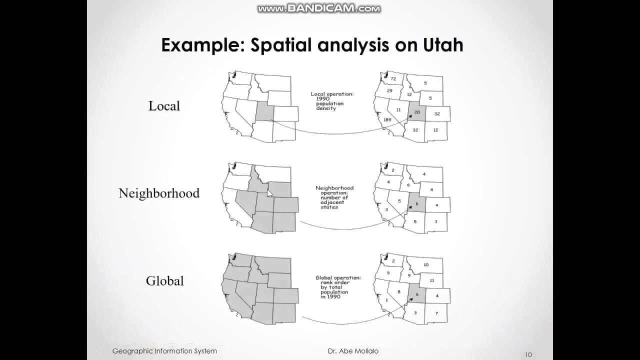 population density of the same state. so that's called local operation. the second type is called neighborhood operation and this operation uses data from both input location plus the nearby or neighborhood locations to determine the output value. so that's why it's called neighborhood operation. for example, let's say: let's say you want to. 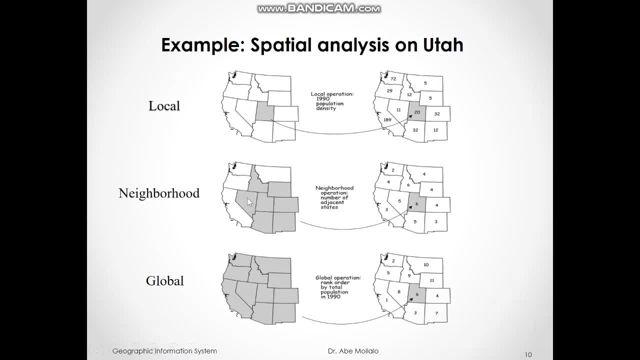 find out the number of adjacent states to the Utah State. okay, or in other words, how many states share boundary with Utah. in this case, we not only consider the location of Utah State, but also the surrounding states as well. to calculate how many adjacent states to Utah State, which is one, two, three, four, five, six and. 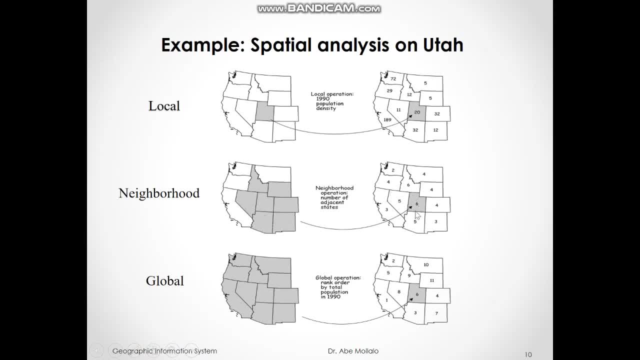 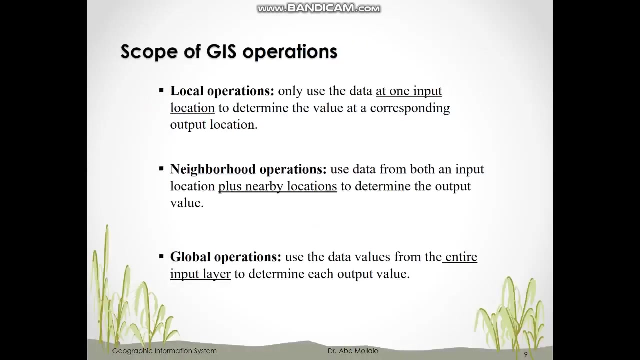 the output will be six right, so that is called neighborhood operation. and neighborhood operation involves neighbors of a study region. from calculation, for example, for California it shares border with one, two, three. so the output will be three and depends on the neighbors. third type is global operation, which 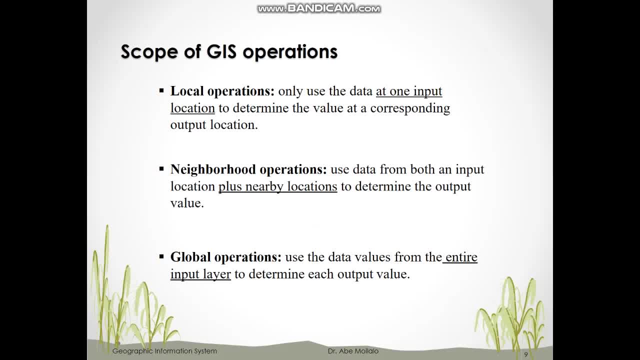 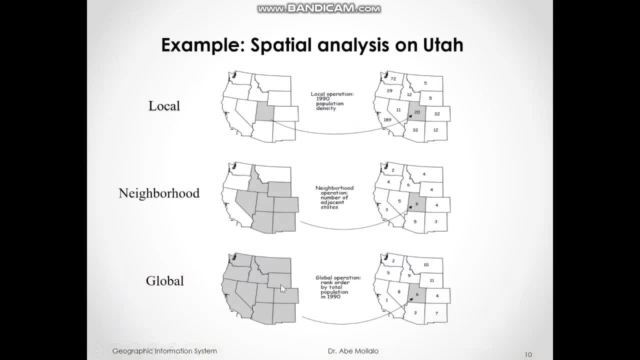 means this operation uses data value from the entire input layer to determine each output value. for example here here is: let's say we want to rank Western states by their total population for the year 1990. in this case we not only consider the population size of, for 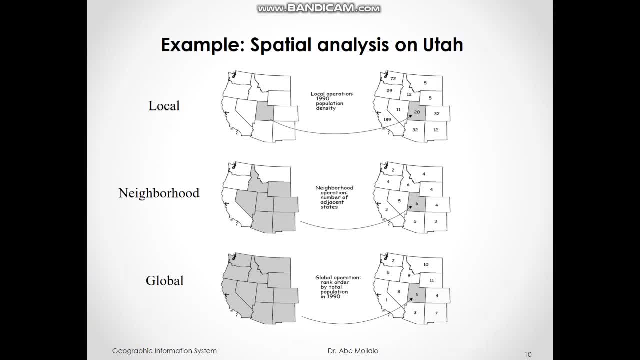 example Utah, but also the population size for all of the Western states, all of this study area, and then we can rank them in order and find out. Utah actually has a rank order of six, okay, and California has the largest population, ranked number one among the other state. the second one is Washington. 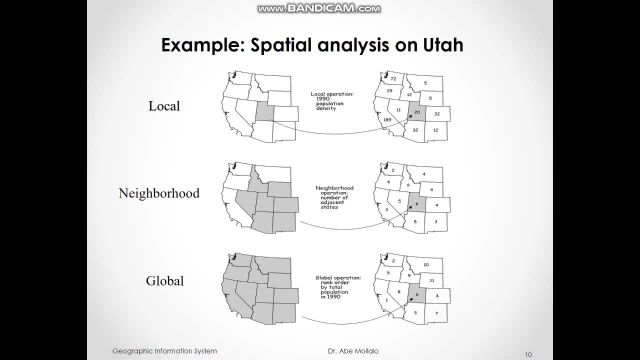 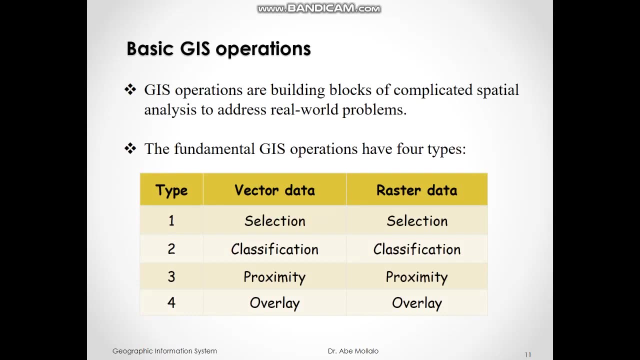 alright, so Route than the other states and the local stateera. all of these it does not mean is the local state is ranked as a priority, so the date of young bikers that face difference somewhere we have one second depend on. Dragunov says that the current observation options are completely. 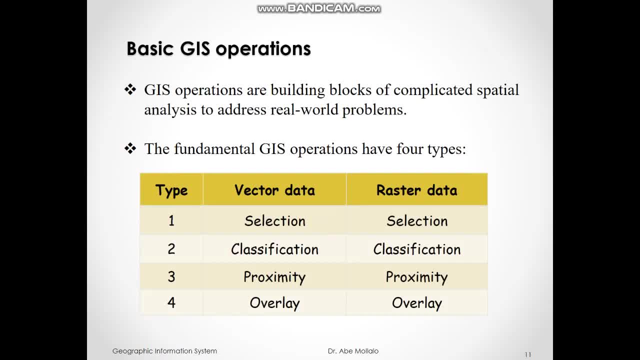 burned out and are being moved, along with a pre-selected simulation system, anywhere it's happening. so, based on the year 2010, the estimation urban areas, as said, and this individual has to understand what the resolution authority is about, and that's why the development policy is in place in favor of operations. 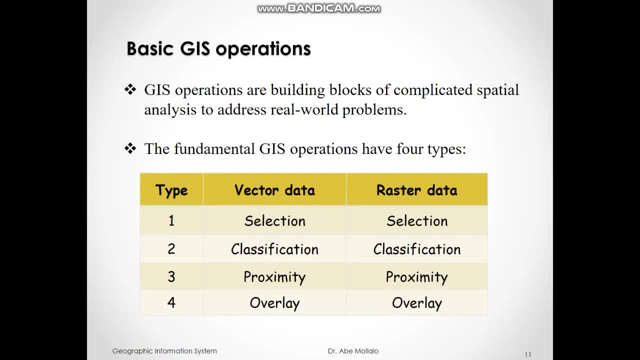 and proximity and overlay, which are applicable for both vector and raster data set. we're going to talk about the operations one by one, and in today's class we will talk only about selection and classification, and proximity and overlay is for the future lectures. let's start with the 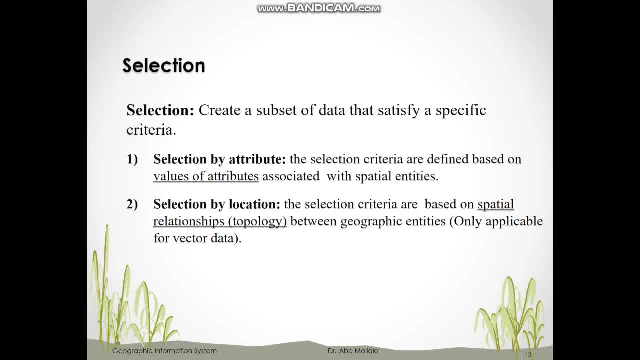 selection. so selection is a GIS operation that creates a subset of data that satisfies certain criteria. so there are two types of selection: selection by attribute and selection by location. selection by attribute: that we already have worked with. we use that to select a specific type of cancer based on location and it's selected specific records or feature based on attribute. 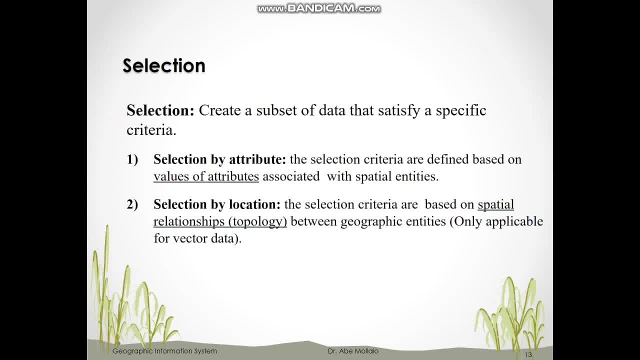 values. but the selection by location selects record based on the spatial relationship like contain, composition, intersection, adjacent or in general a topological relationship that we talked about before. So selection by location is only applicable for vector data model, because raster data do not have any spatial topological information. 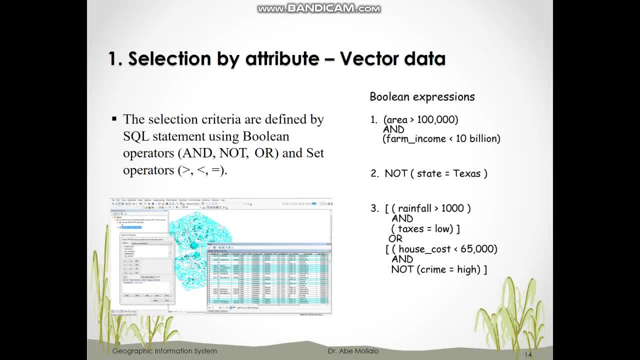 So let's start with the selection by attribute for vector data. There are a number of operators you can use, like and not, or greater than less than equal to, and so on, to write your statement or query. So you can use these operators to build the query statement to set to specify the selection. 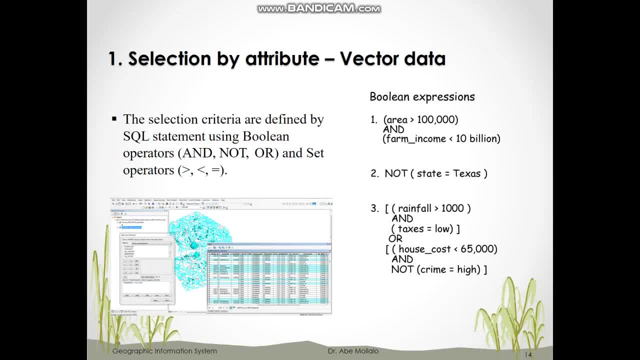 criteria. So you can use these operators to build the query statement to set to specify the selection criteria. So you can use these operators to build the query statement to set to specify the selection criteria. So we've worked with that in the previous labs. So basically in select, 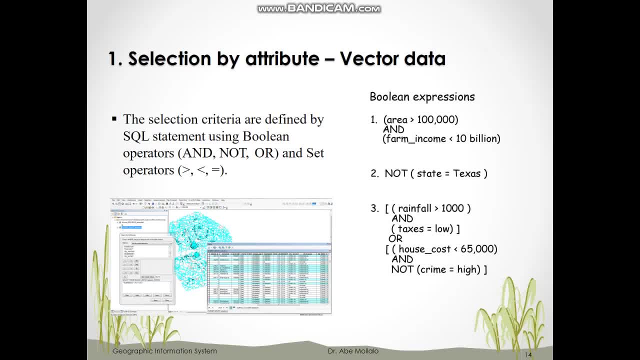 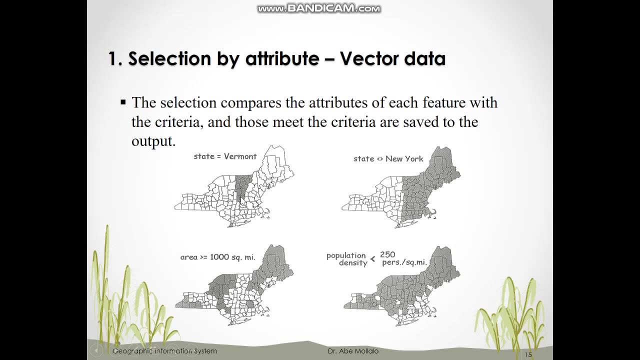 by attribute. GIS applies the query on each feature and then compares the attributes of each feature with the criteria. The feature or records that meet the criteria will be selected. For example, here we want to select all counties with attribute name of the state of Vermont. 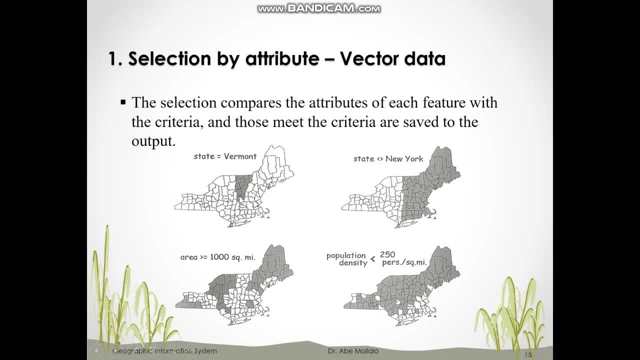 So it is based on the attribute table. or we want to select all counties that their attribute name is not New York, So this operator is shows not, and. or we want to select all counties with areas larger than or equal to 1000 square miles, So you can see that. so it's based on the 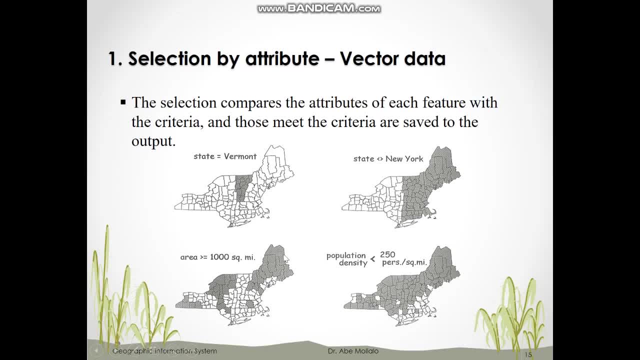 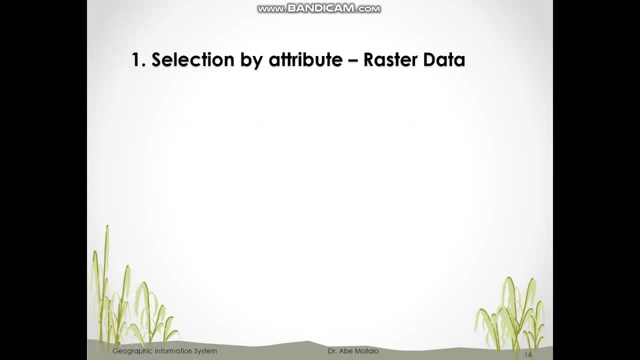 area Based on the attribute table. there is a field with the name of area, so based on that one we can select all counties or select the counties that population density is less than 250 percent per square mile. So these are the selected counties. Selection by attribute can also be applied to. 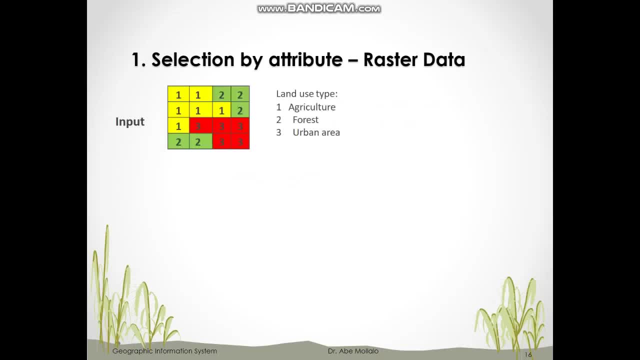 raster data. So let's say we have a very simple raster data set which describes land use type for a study area. One represents agriculture, two represents forest and three represent urbanized area. Let's say we want- we only want- to tease out the urbanized areas. okay, We can define the SQL. 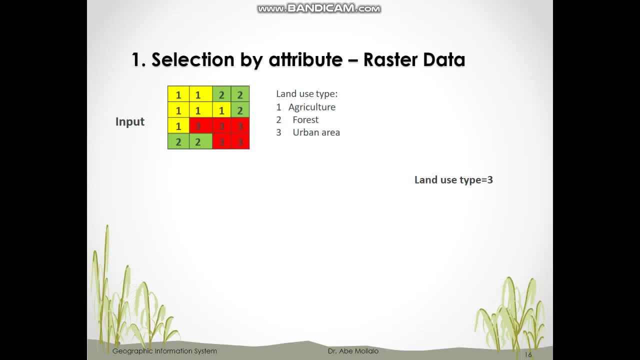 statement like land use type equals to three. and then GIS will read this criteria and then compare that compared every single pixel, one by one. So let's start with the first cell. The first cell is one and one doesn't satisfy the criteria because land use type is not equals to three. So the output: 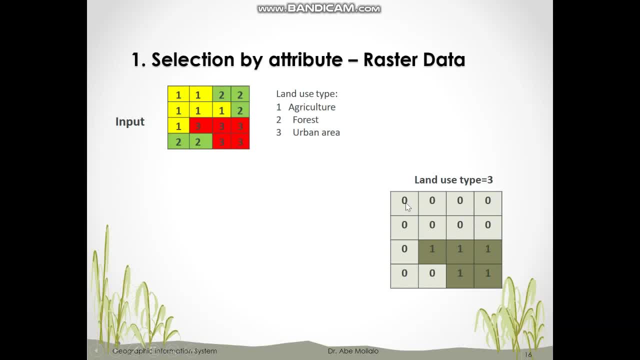 will be zero, which means false. and then we go to the next cell. The next cell, again, is one and doesn't satisfy, so zero. The third one is two and doesn't satisfy is not three, so zero. So until we reach this cell. this cell is three and three. land use type is urban area, so it satisfies the criteria. 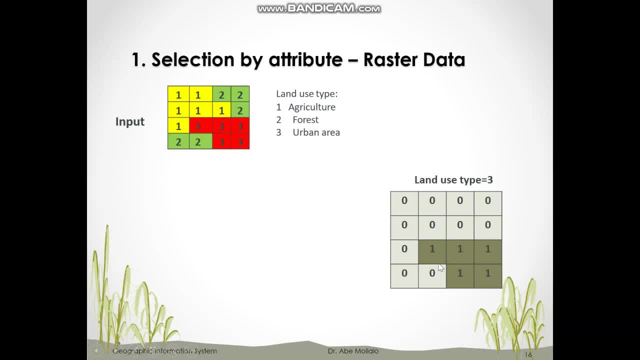 So the output will be one. So one means that criteria is satisfied, and so that's how GIS, that's how computers can scan and do the select by attribute for the raster dataset. okay, so keep in mind that the output of selection by attribute for raster dataset is always a binary grid. It's always either zero or one. okay, or how. 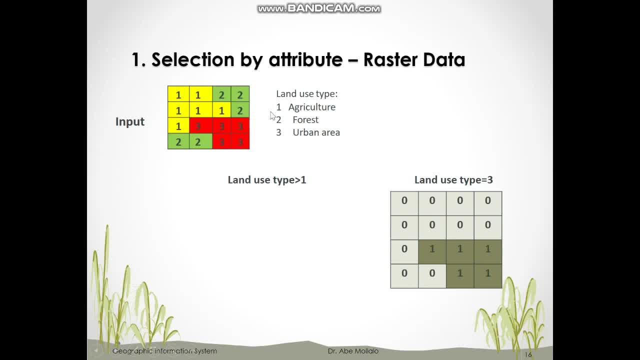 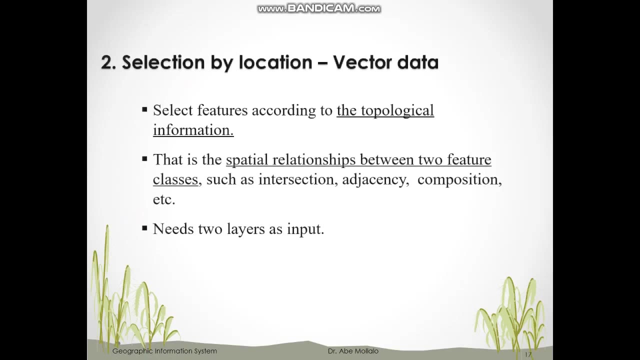 about this: one Land use type greater than one. so it compares each cell to the criteria, and if it satisfies the criteria the output will be one, otherwise it will be zero. so again, the output is only binary raster. so let's move on to the second type of selection, which is selection by location. so here, 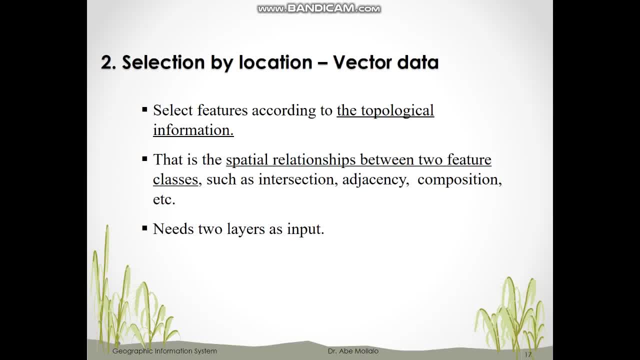 our selection criteria is not defined based on attribute information. it's defined based on a spatial relationship or topological information. spatial relationship between two features we have talked about before include the intersection of two lines or adjacency between two polygons, or composition of polygon, or line or containment. so these are a spatial relationship and selection by 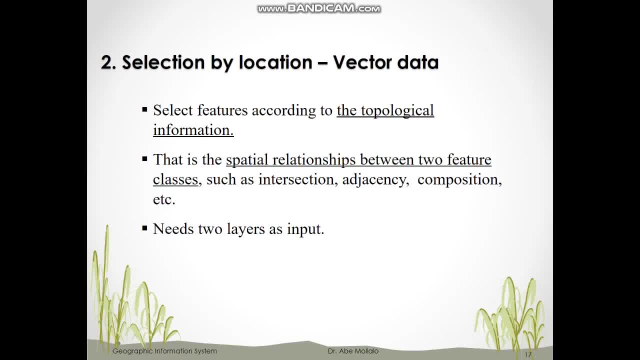 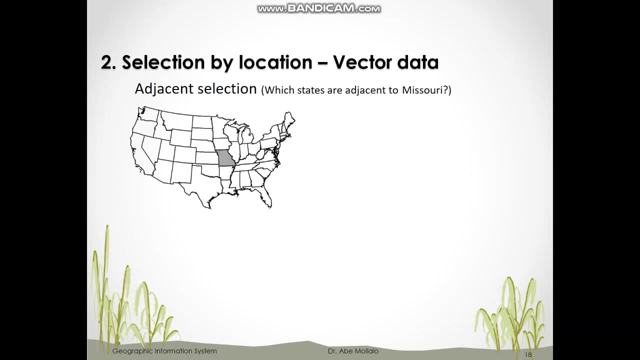 location usually involves two or more layers as the input, so we need at least two layers for the selection by location for the vector data. let's see one example of selection by location based on adjacent selection. so we want to know which estates are adjacent to Missouri, and so we have a shape file of Missouri and a shapefile be all of the US states. now we're not. 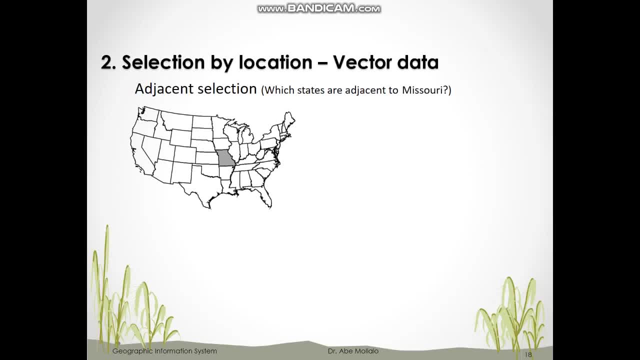 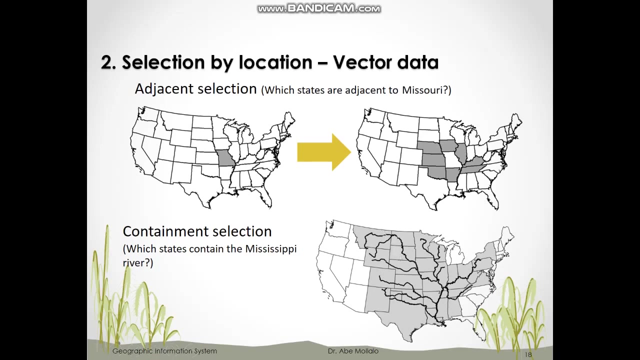 looking at attribute of the Missouri estate, but we look at a spatial relationship between Missouri estate and the surrounding states, and then the surrounding polygon can be teased out like this. so our containment selection is another topology relationship. for instance, which states contain the river, so this is the Mississippi River, okay, and and we have it as a shape file. 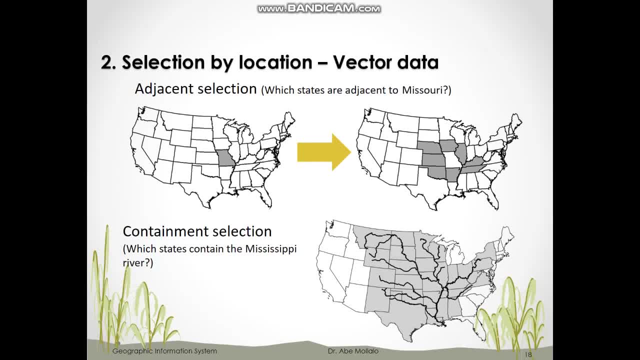 and also we have used US states as another shape file and all states that contain part of Mississippi River, the entire state will be selected out. so these gray states, okay, all of these gray states, they contain part of Mississippi River. so in selection by location, we're looking at the spatial relationship. 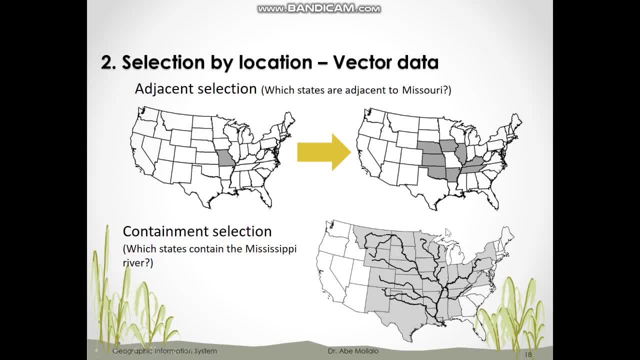 between the features, for example, adjacency or containment, sometimes it's intersection, sometimes it's composition, so this is called selection by location. we're not looking at the attribute table, but we're looking at the relationship between the features, and ArcGIS provides a user-friendly interface to help us to. 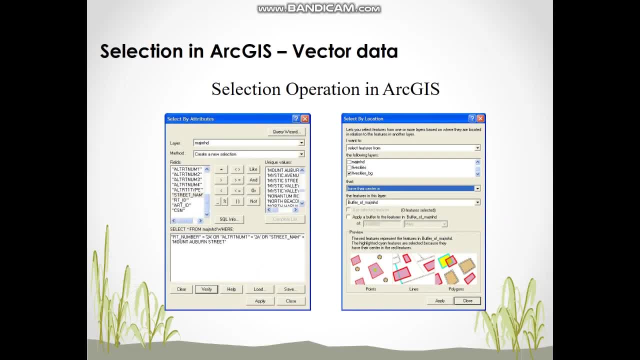 construct SQL SQL statement to specify selection criteria, and this dialog helps us to define how to select features based on the attribute or based on the spatial relationship. so here is select by attributes and here is select by location. we already have worked with select by attribute and in this lab we 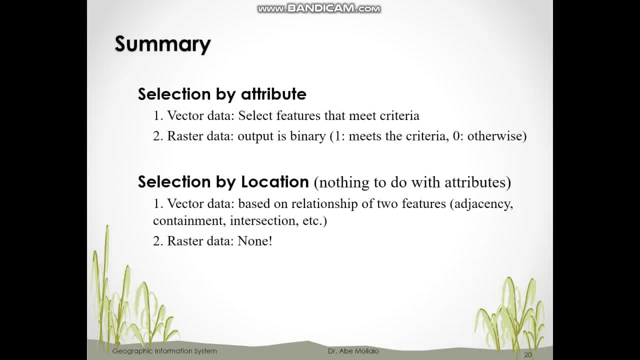 will also work with select by location. so, in summary, for select by attribute for vector data, we apply the criteria on each feature. if the feature satisfies the criteria, it will be selected. and select by attribute for raster: we apply the criteria on each cell, each pixel, and if the feature satisfies the criteria, it will be one. 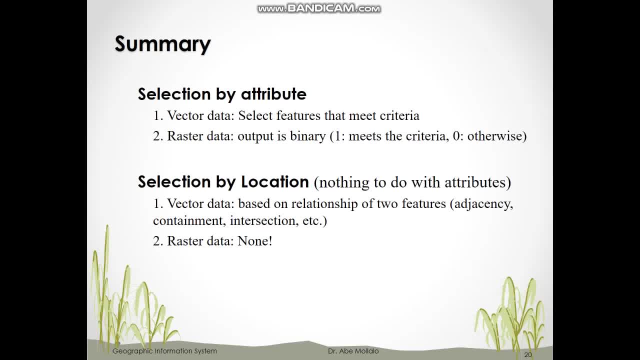 otherwise it will be zero. and select by location has nothing to do with the attributes. it's only applicable for vector data set. it cannot be used for the raster data set because it's based on the relationship or is based on the topological relationship, and topological relationship can only be defined for the vector data model, not for the. 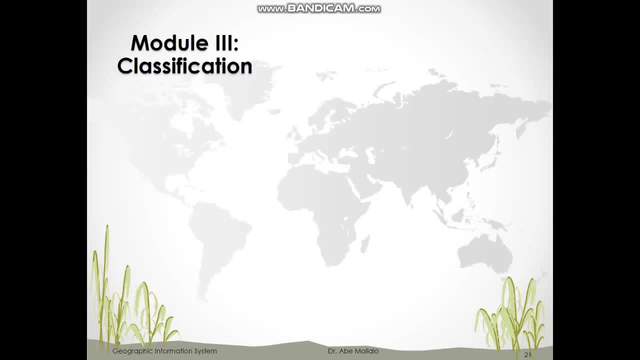 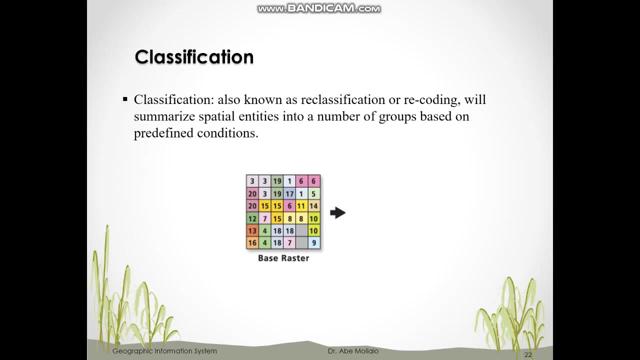 raster data model. another widely used GIS operation is classification. classification is also known as reclassification or recoding, and this operation will summarize the features into several groups based on predefined conditions. so let's say we have an input raster layer and we want to simply use new values to replace old values based on a predefined 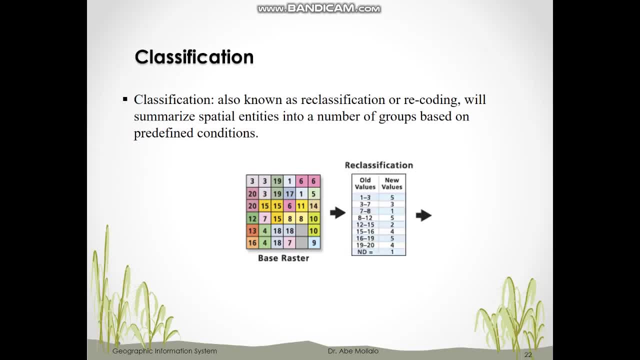 condition, and here is a lookup table, and lookup table basically defines how old values will be replaced by new values. all values between one to three will be replaced by five, and all values between three to seven will be replaced by new values, and so on. so, for example, first cell is has the value of 3, which is old value. 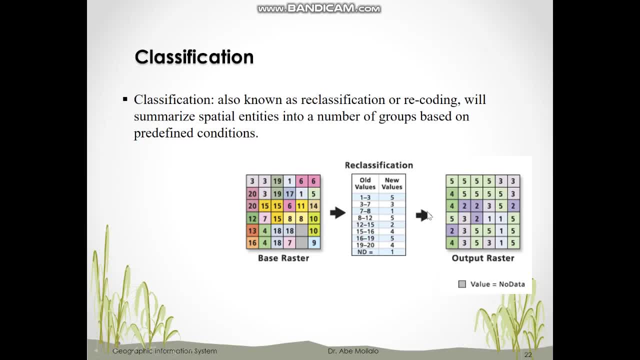 then you look up, look at the lookup table. the cells file falls into this category, right? so the new value should be 5, okay, in the output and output will be saved as 5 here for this cell. and if you look at so, the second one is also. 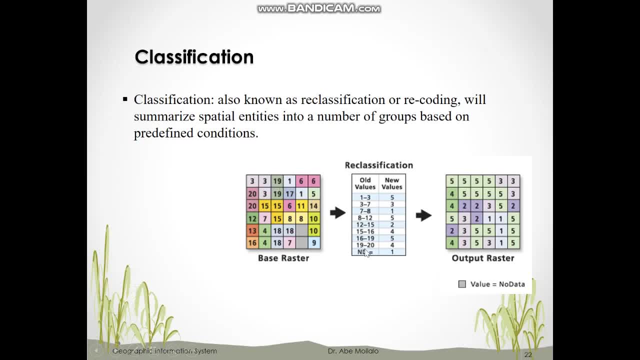 the same 5. the third one is 19, and 19 falls into this category and the new value for this value for this, for 19, will be 5 again. so we can continue this process for every single cell, one by one, to reclassify this image. okay, so this is. 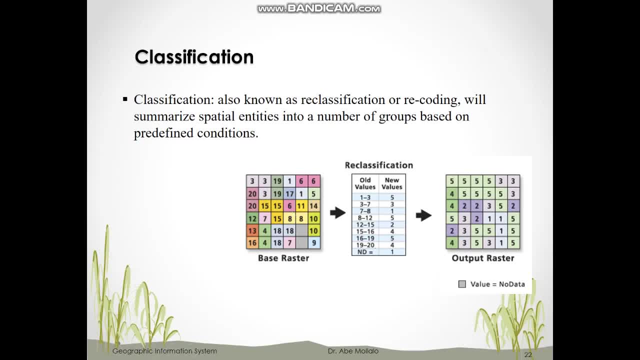 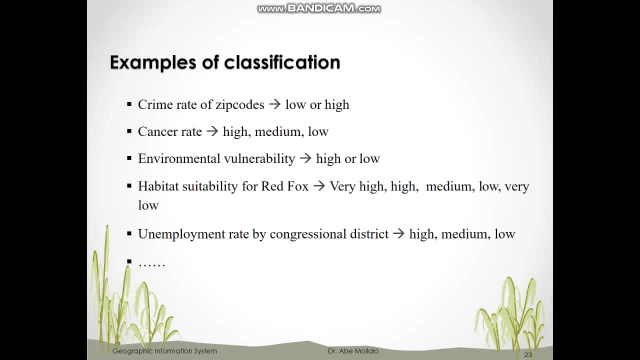 called classification or reclassification process, which is widely used for summarizing and displaying data sets. so you there are many examples or applications for classification. for example, we can classify zip codes into low crime rate, high crime rates. so two categories. we can summarize cancer type, such as brain cancer, into medium, high. 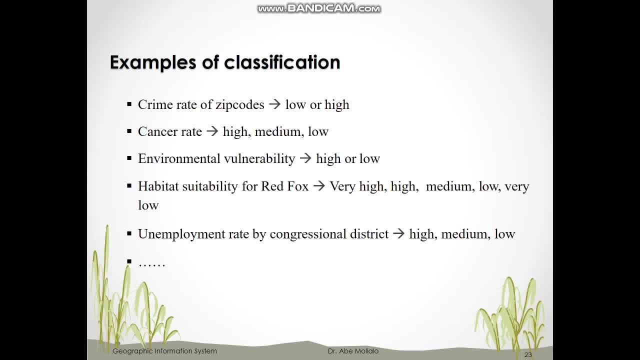 and low rate of the cancer. or we can summarize habitat suitability for red fox to very high or very low rate of the cancer. or we can summarize habitat suitability for a high, high, high, medium, low, very low suitability. so you can see there are numerous applications for classification. so now let's talk about 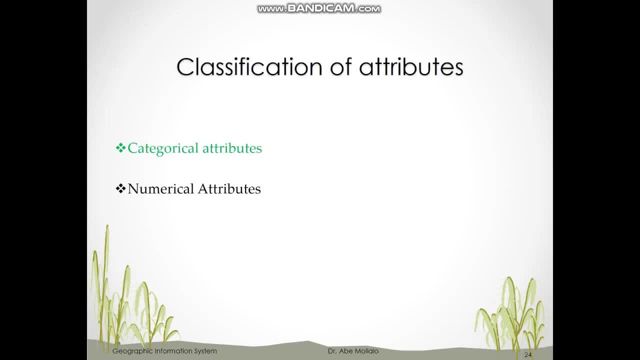 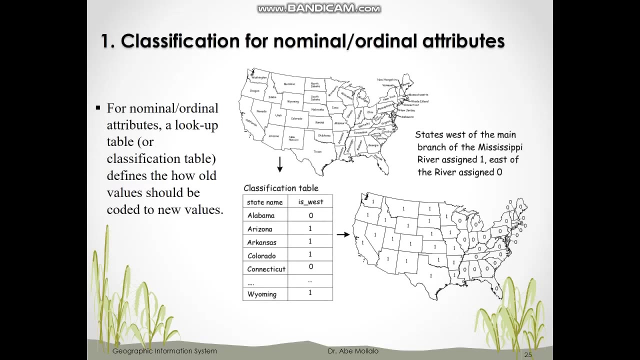 classification for all attribute size. we have talked about different types of attributes before, which were nominal, ordinal, interval and ratio. so we start with nominal and ordinal attributes. nominal and ordinal attributes are also referred to as nominal, odd and ordinal attributes and thank you for your attention. and if you haven't seen one of our series of 5 Magazin at the top example: 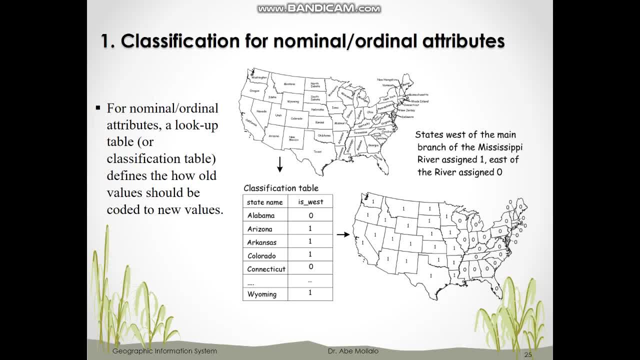 here. organised applications are in the description down there you can find these categorical, variable or categorical attributes. for classification of categorical attributes it's very easy. we should use a lookup table for classification like this, and lookup table basically defines how old values will be replaced by new values. for example, let's say we're going to recode. 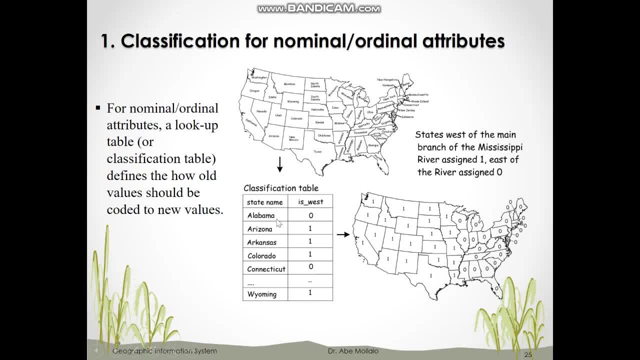 all the states in the West of main branch of Mississippi River as one and and all the states in the East of River as zero. so here is the classification table. old values are categorical values, right? so these are just names, and new values are specified as either 1 or 0. so here is the classification results. okay. 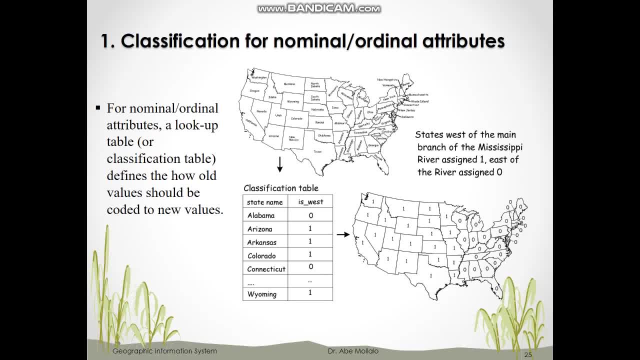 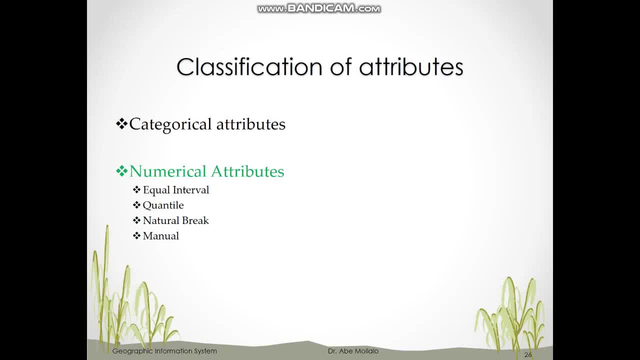 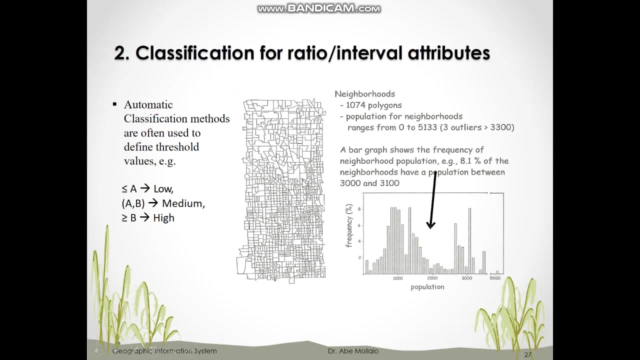 so that's for categorical attribute, summarize or group the data. now let's uh move on to the interval and ratio attributes, which are also referred to as numeric attributes, which is more sophisticated. so, for example, let's say: we have a study area, this is this is our study area. this is a community with more. 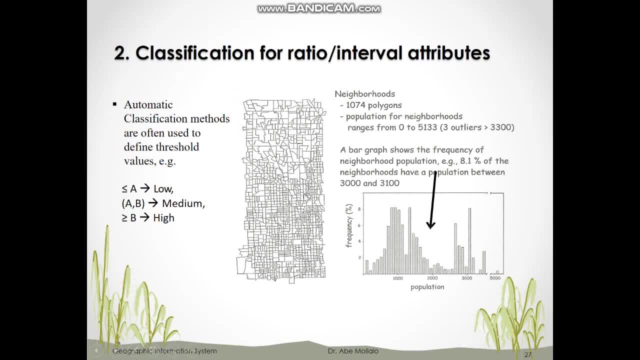 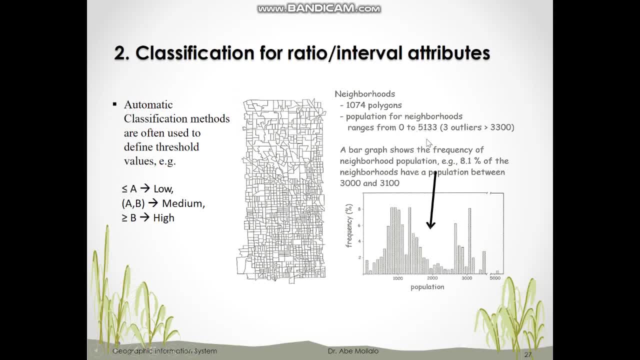 and let's say we want to reclassify our city area into 3 categories based on population size, to low, medium and high population size. and 3 categories mean we need to define or determine two cutoff values: okay, A and B. so below A is assigned to low category, between A and B and B platen as 3 category. then we have to change it to a lower category between A and B and we have to change the pot05 is assigned to lower category between A and B, and then we have to change the ratio of value to lower category between A and B and then we have to change the value as you gozer. 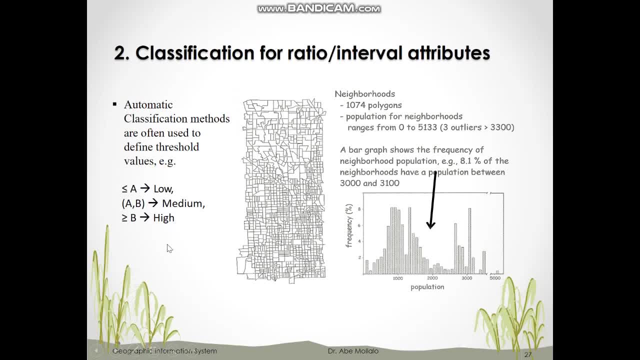 before categorization: change to low category between A and B and we're going to accept some score of a third category. the total character is important a on. again, if data numbers and polygons will be assigned to the medium population size and above B, we consider that consider this polygon as high population size. so question is how to 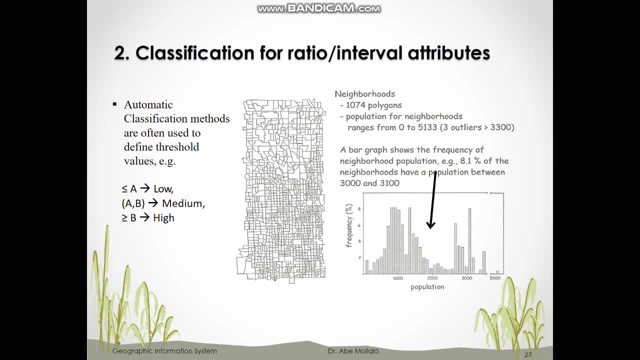 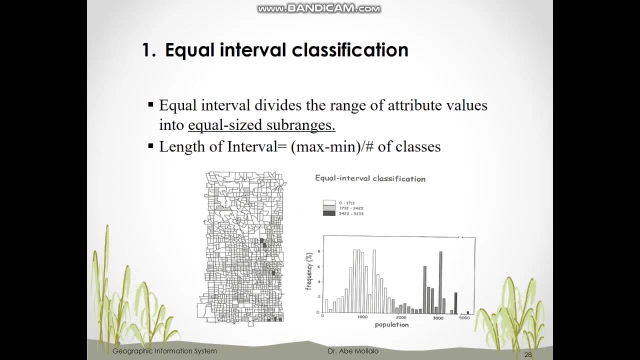 determine the cutoff values A and B? and the answer is we need some automatic classification method to help us to determine or define threshold values. there are a variety of ways for classification, and the first method is called equal interval classification, which means the range of each category is going to be the same, or equally split the range from 0 to 5000 and 133, which 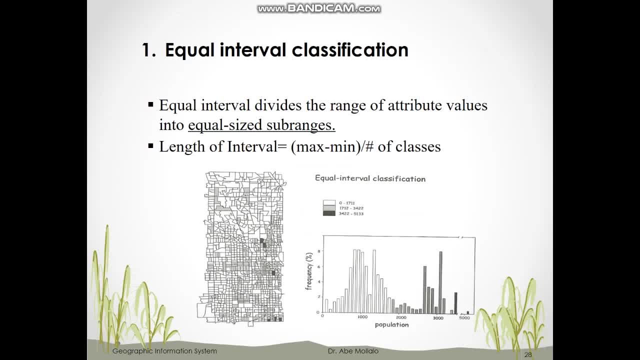 is the maximum population. so you can see the entire study area is divided into three categories and from low with white color, medium with gray color and high with black color. and if you look at the range of each category, from minimum to maximum, ranges of each class or category is equal. that's called equal. 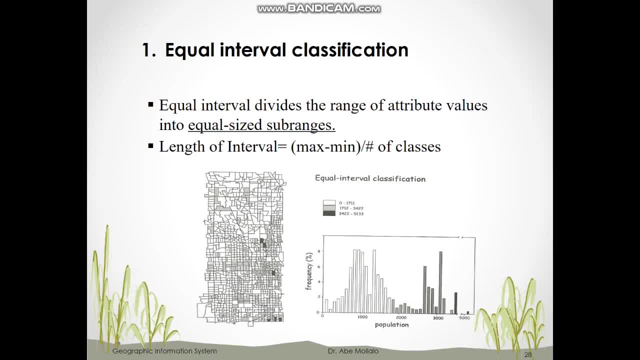 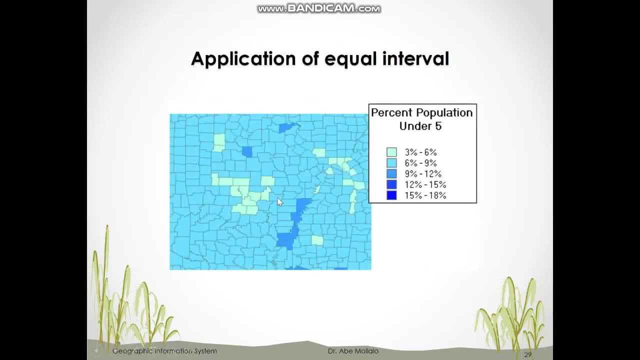 interval classification. maybe this picture is not really clear, so let's see the next picture, the next slide, that percentage of population under five so has been classified into five categories. and when you look at the ranges, the ranges are between three to six, six to nine, nine to twelve. 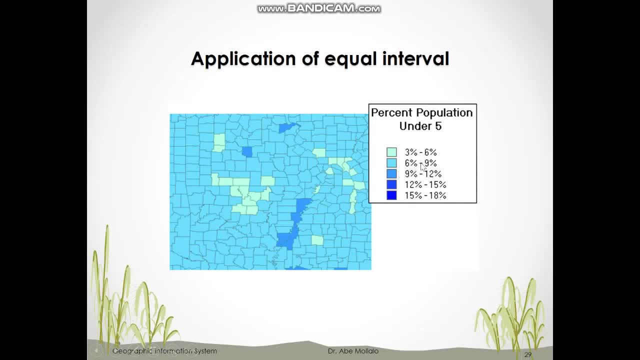 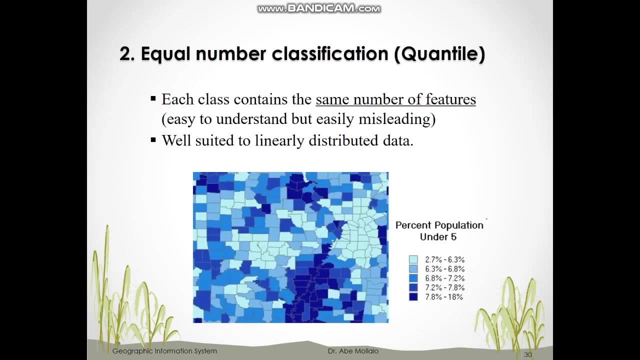 to fifteen, fifteen to eighteen, so the ranges are equal or they have equal interval. okay, so that's the first type of classification. the second method that helped us to determine the cutoff value is called quantile classification. so in this classification method the threshold or cutoff values are set. so 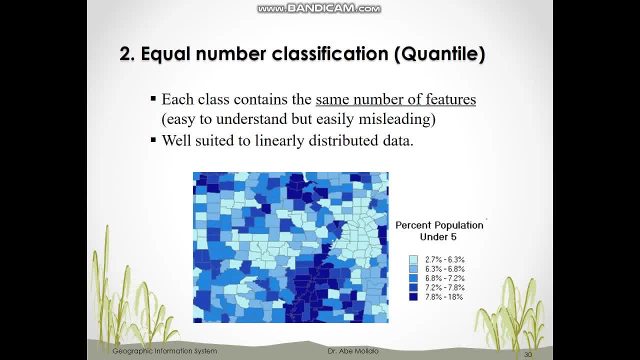 that each category is going to have the same number of spatial features. spatial features: the same number of features, for example, in this color and the same number of features in this color, and so forth so on. so this classification method is suitable for linearly distributed data. so you can see. 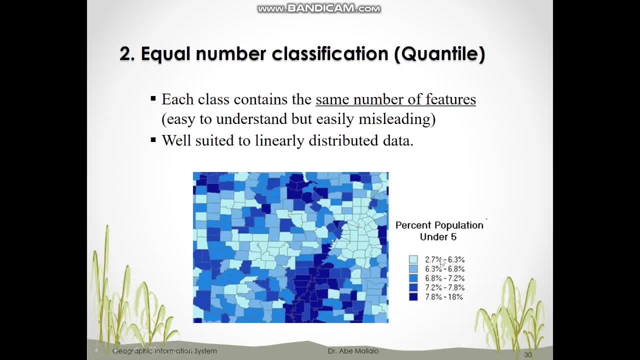 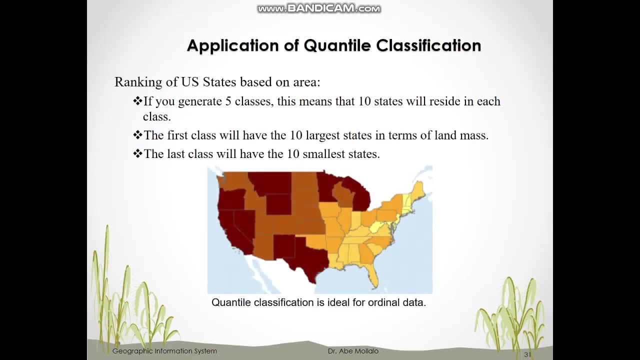 the categories will have. however, the range for each categories are different. within each category, the number of features is almost the same or the polygons are approximately the same. that's called equal number classification or quantile classification. so let's see an application of quantile classification in GIS. for example, we want to rank US. 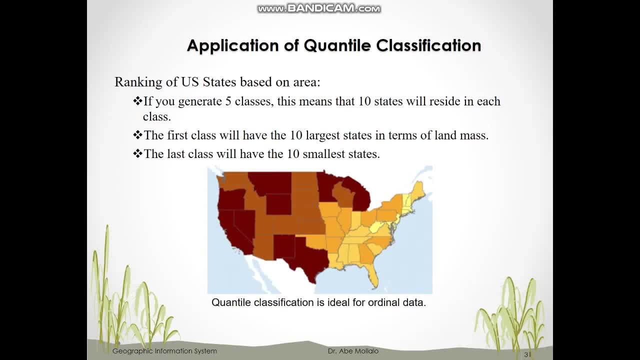 states, based on their areas, into five categories, so we use quantile classification. if you generate five classes, this means that ten states will reside in each class, each class. the first class will have the ten largest states in terms of landmass, and the last class, or last category, will 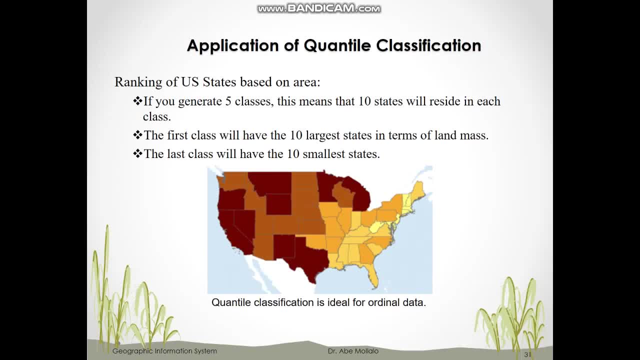 have the ten smallest states in terms of landmass. so when you use the quantile map classification with five classes, it will look like this map. so it is easy to see see that it is easy to see that states like Texas or California or New Mexico are in the top ten for landmass. the 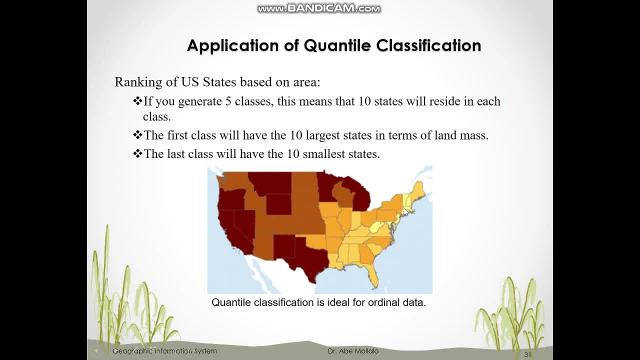 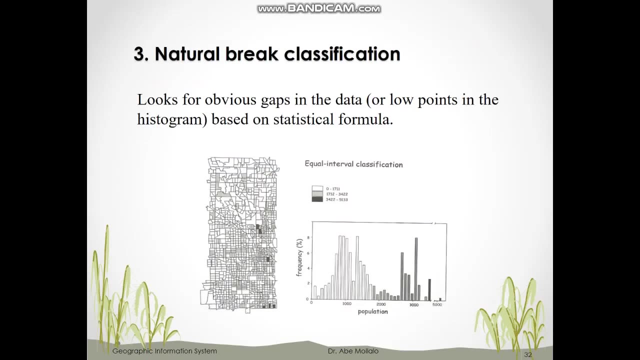 east coast states are obviously the smallest, so quantile classification is ideal. when there is an order in the data is suitable for ordinal data. and third method that helps us to determine the cutoff value is called natural break classification and this might be the most widely used classification technique. 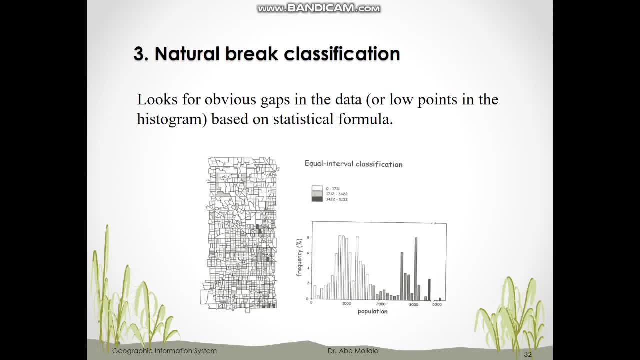 this classification is based on the histogram and looks for the obvious or gaps in the data. so let's say, in the same study area, this is the histogram of the same study area and x-axis indicates population size from 0 to maximum, which was 5133, and the y-axis tells us the frequency of the occurrence of the. 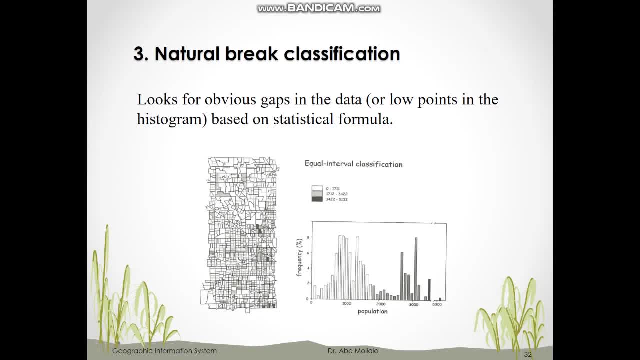 population, which means number of polygons you have for this population size. then if you look at the histogram of the population size, you can see that the histogram here we can identify the number of natural gaps. for example, here is a gap and also here is another largest gap in the data. so the natural 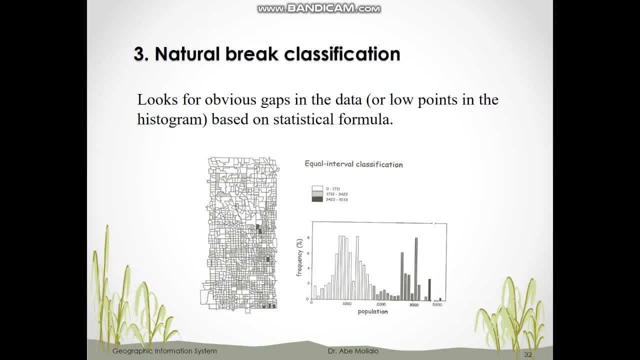 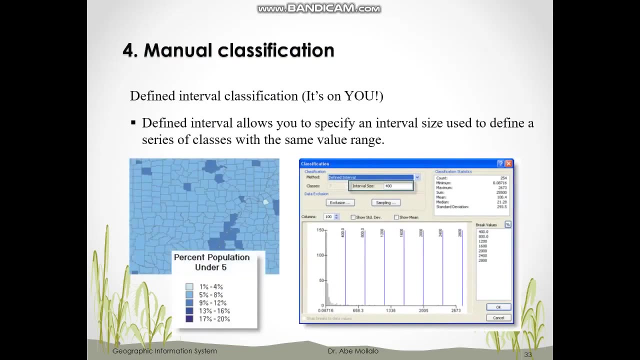 break. classification uses mathematical formula to help us to find the largest gaps in histogram and then we use these gaps as cutoff values. so technically it minimizes variance within each class and maximizes variance between the classes. the last method is called manual or defined interval classification method. so the 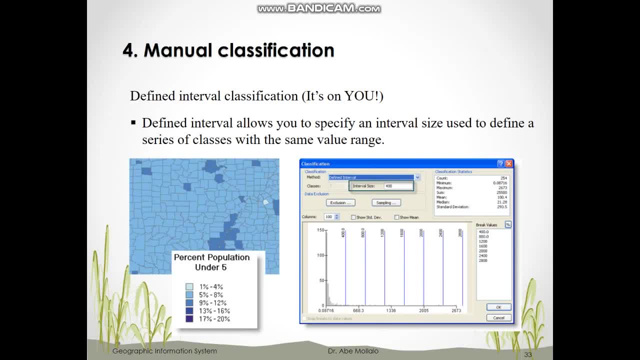 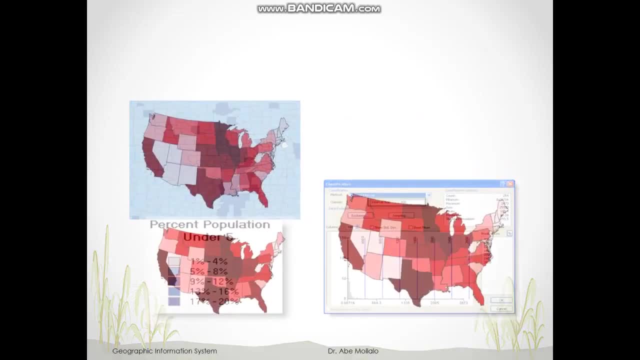 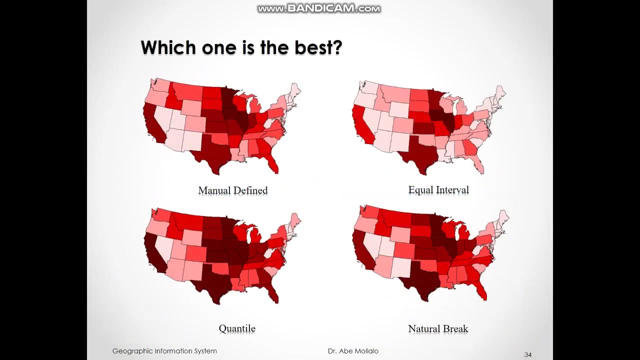 choice of cutoff values is up to you and you define intervals or cutoff values. so we talked about four different type of classification method for numeric attributes: manual, defined equal interval, quantile and natural break. so you can see: for the same data you got different visual results or different pattern. 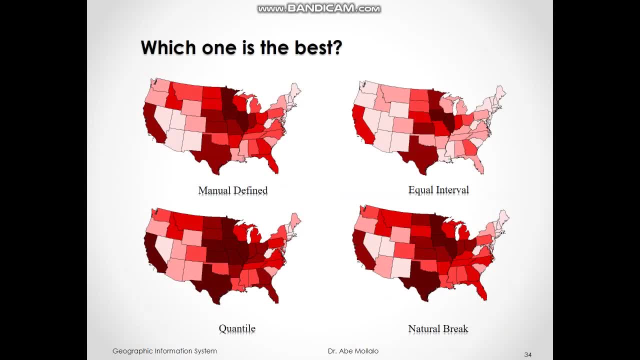 that's why people say maps can be misleading. if I change cutoff value for each class, I will get different result. if I change the classification technique, I will get different results. so the question is which one gives us the best display of data, and here are some criteria or guidelines for you to select. 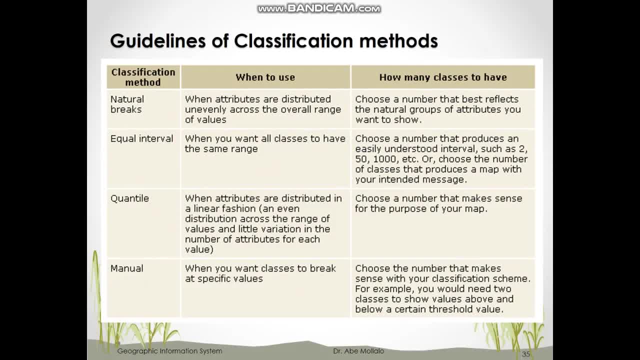 the best classification method. so you always have to be very careful when you choose the best classification method, so you always have to look at the data when. when do we use natural break? so we use natural breaks when the attributes, like- I don't know- population size- are. 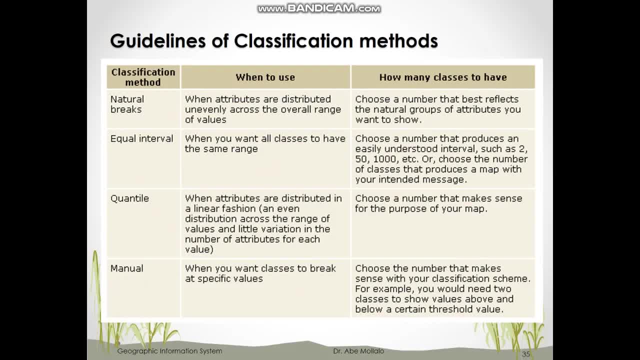 distributed unevenly across overall range of the data. so then, when you look at the histogram of the data, you will see some pics. the distribution will be like this, and in that case natural breaks might be the best choice. so you choose numbers that are equal to the distribution of the data, and then you 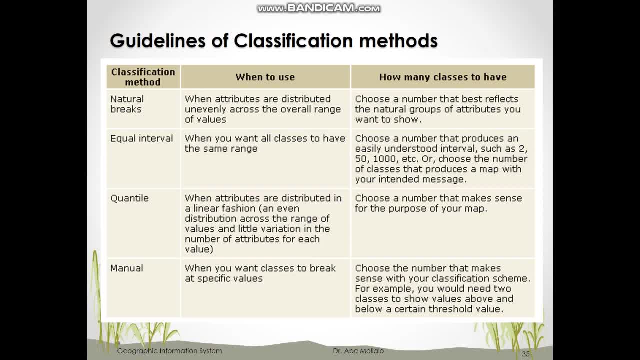 choose that best reflects natural gaps within your data. and how about equal interval? equal interval classification is suitable when you want to have all classes with the same range, for example, if you want to display categories for every 1,000 increments and then interval is 1,000 for every category in that case. 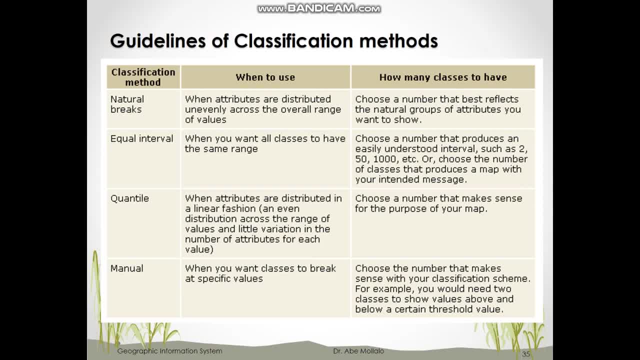 equal interval is suitable. the quantile classification basically means that the same number of the geographic feature for every category, and the best time you can use this classification is when you when your attributes are linearly distributed across the range, which means that if you draw out a histogram, 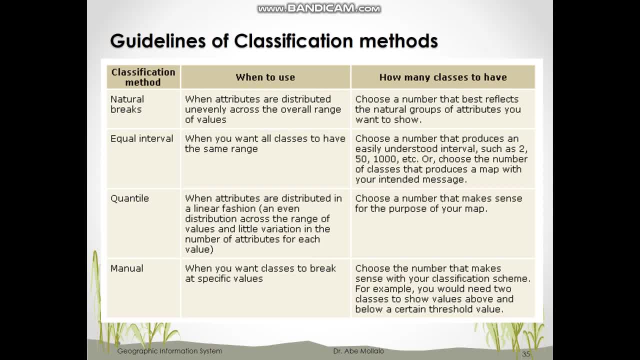 there is no pic, or basically it's flat for histogram or probably there is a very. it has a very gentle slope and the manual classification and the manual defined classification can be used when you want your classes to break at a specific values. so that's the guideline for classification method. so 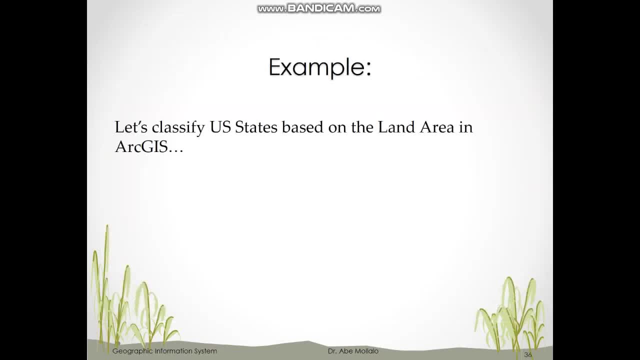 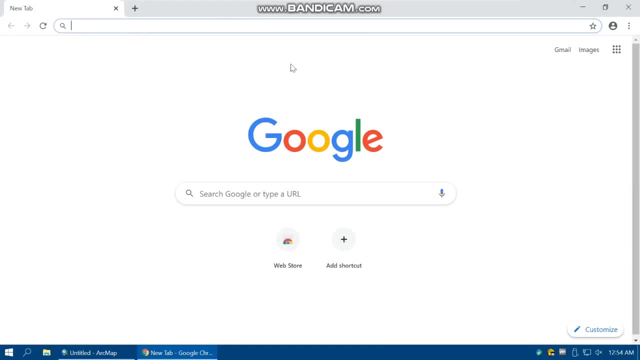 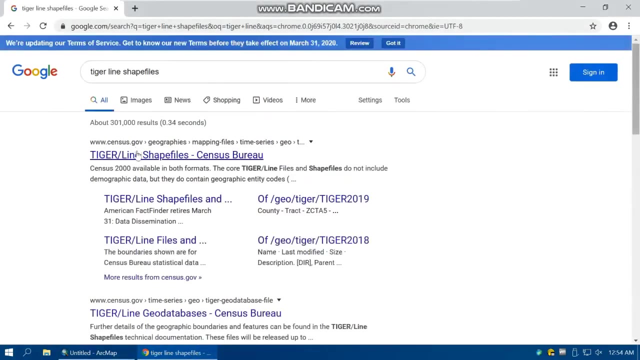 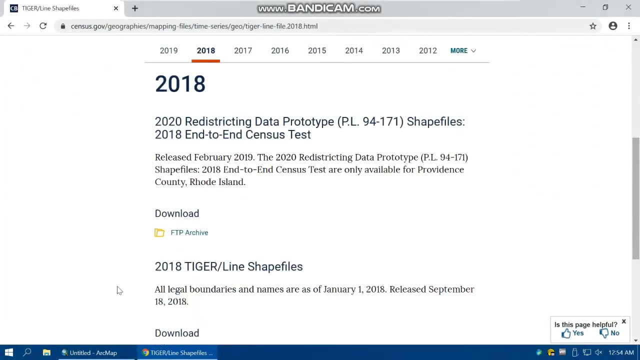 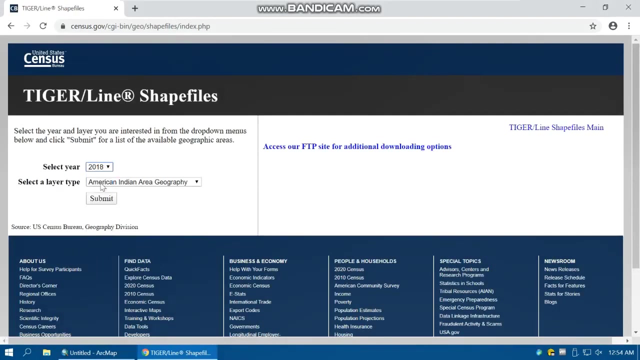 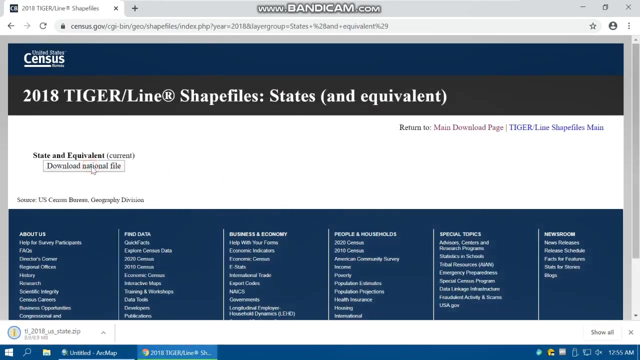 let's open up ArcGIS to show you classification techniques. first of all, we need to download you as a safe boundaries from tiger line. so if I here type tiger line and then go to the tiger line website, the most recent data web interface and states and equivalent submit download national file. 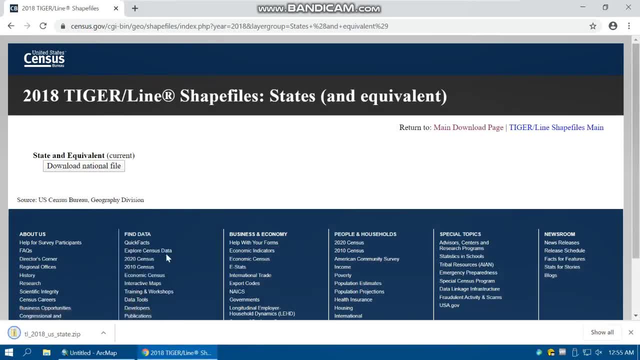 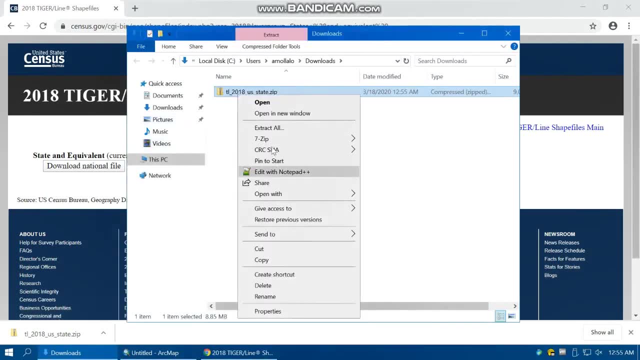 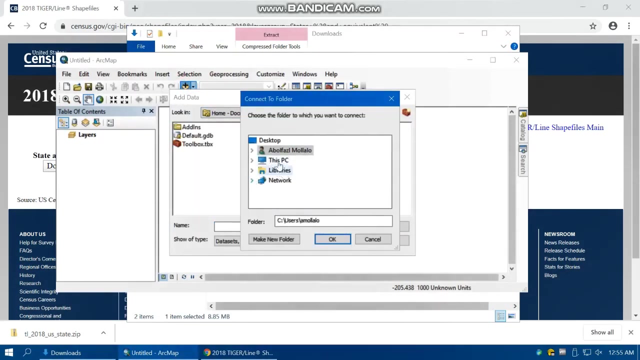 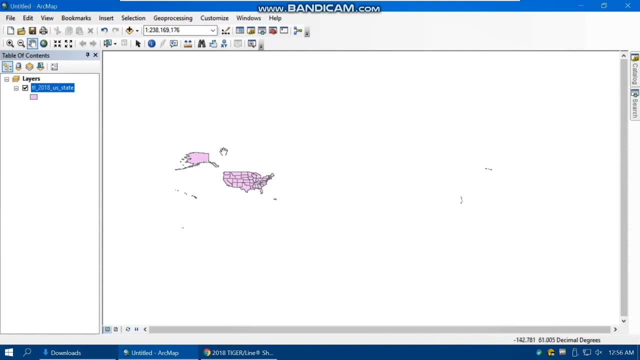 and then let's extract it to the file and load it into ArcGIS. and load it into ArcGIS. we're going to classify- yes, shape file based on the land area. so just click on command key and now you can see everything it takes to do this class the. 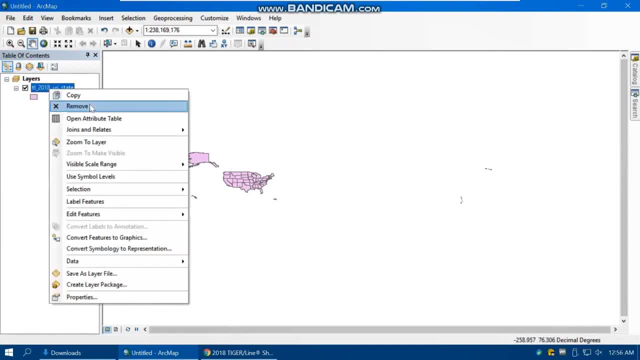 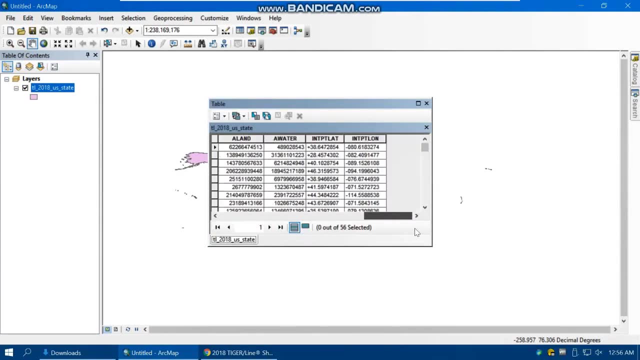 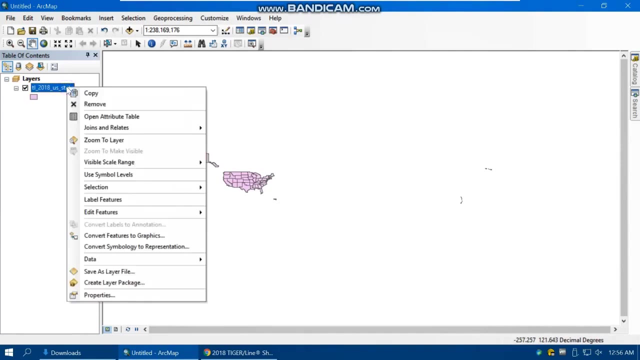 since this will take two minutes to take care of the class file and so you can see. so if you open our attribute table of the estates, there is a field with name of a land. I think this area land and I'm going to classify it based on the